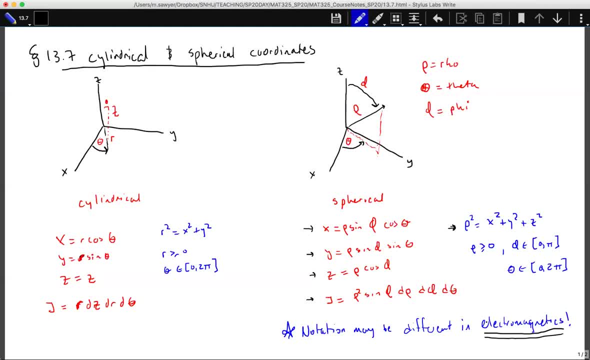 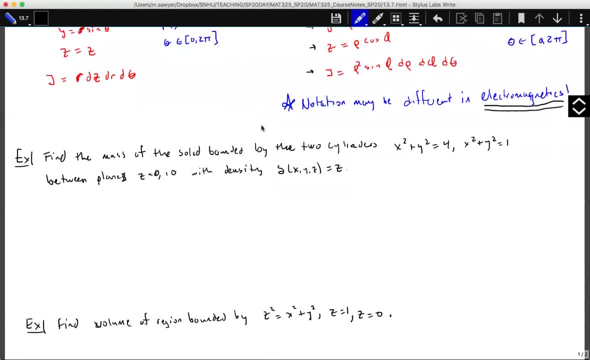 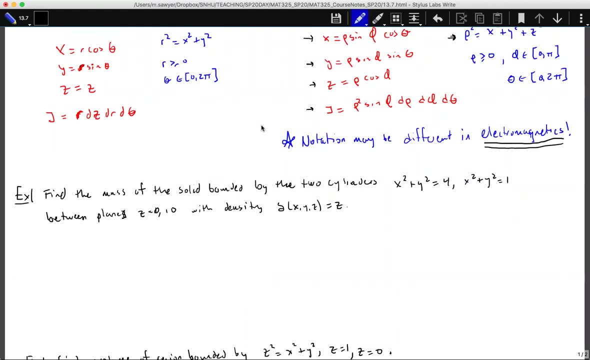 this course. It may be different in different engineering fields, so please keep that in mind. So let's go ahead and start working examples. So let's find the mass of a solid bounded by two cylinders. So let's suppose that we have cylinders x squared plus y squared equals 4, and x squared plus y squared equals 1. between the plane z. 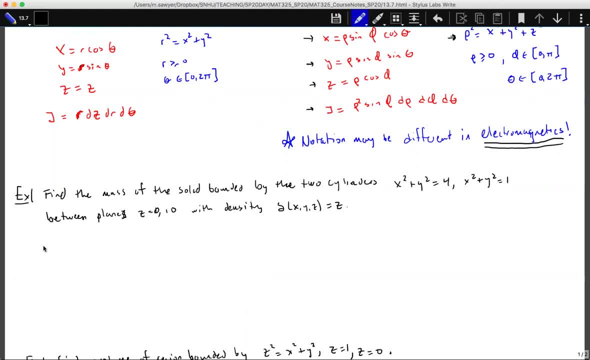 equals 0 and z equals 10 with a particular density. So if we set this up we can look at our kind of diagram here. So on the x-y plane we have our cylinder with radius 1 and we have our cylinder with radius 2.. And so we're looking at our 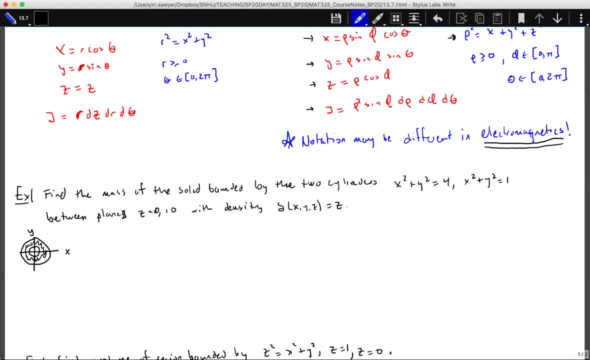 projection where, if we think about z as projecting out of this board, we're looking at the area between these two cylinders, And so, if we think about this as two circles, our radius goes between 0 and, excuse me, goes between 1 and 2.. 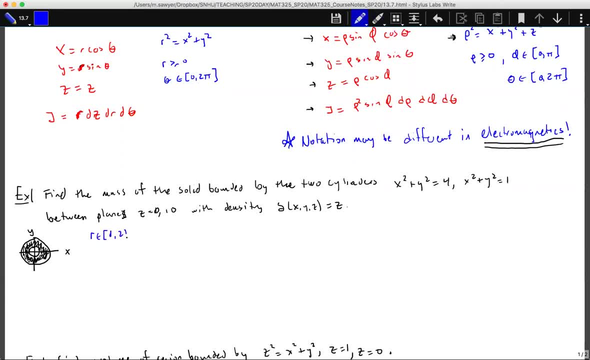 We also have the edge of our circles, So radius goes between 1 and 2.. Our theta goes around the circles, so between 0 to 2 pi, And our z goes from the height of 0 to 10.. So using cylindrical coordinates makes it so we don't have to worry about. 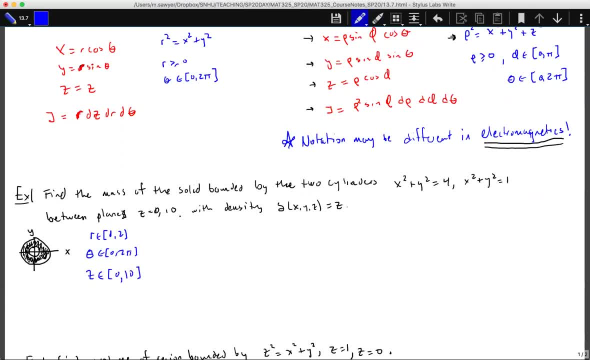 any square roots for our x and y functions. So then we set up our interval here, we set up 0 to 10.. 0 to 10, or we can set it up in any particular order, so long as we're careful with our notation. 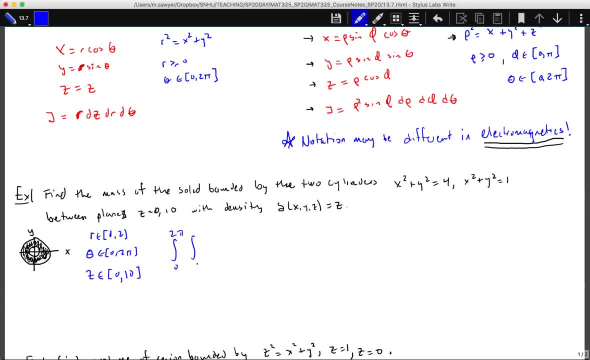 but let's follow our jacobian 0 to 2 pi, 1 to 2, and then we have 0 to 10, and then z times our jacobian r dz, dr d theta and so z. so we get 10 squared over 2. so let's see 0 to 2 pi. 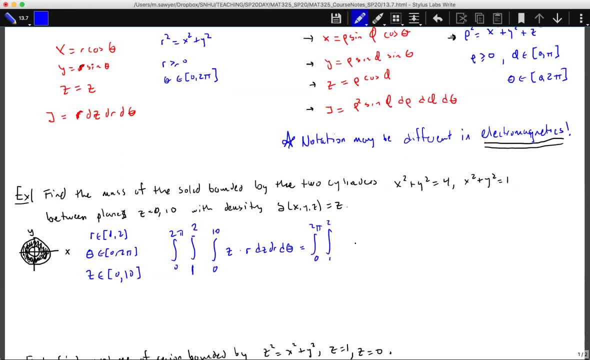 1 to 2, so z squared over 2, so that gives us a hundred over 2, which is 50 r, dr d theta. so now we get r squared over 2, so 0 to 3 pi, so R squared over 2, so that's 25 times 4 minus 25 times 1 d theta. so this: 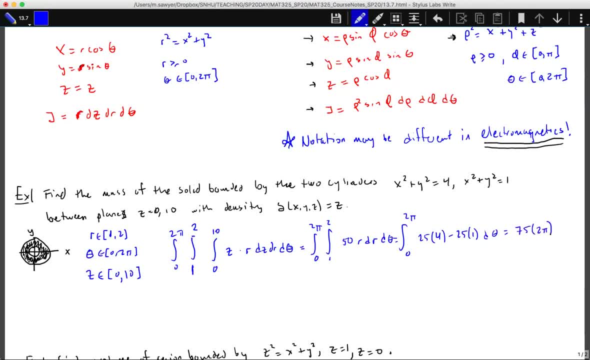 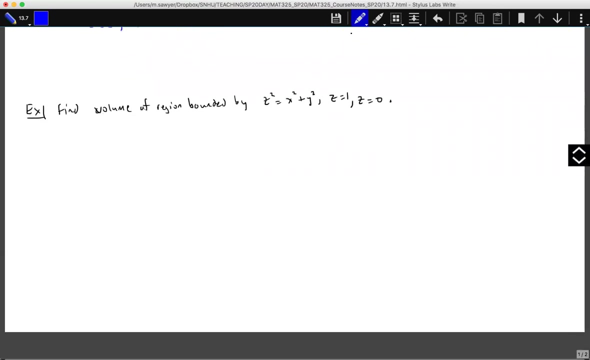 gives us 75 times 2 pi, which gives us 75 times 2, is 150 pi, as the area between these two, of this particular solid with this density function. so let's look at another example here. let's find the volume of the region bounded by these. 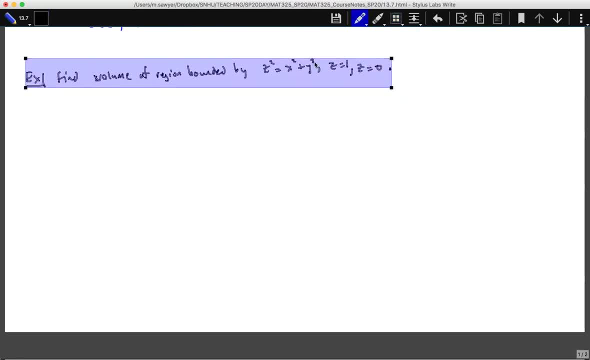 particular surfaces. so we have z squared equals x squared, plus y squared, z equals 1 and z equals 0. so this looks like a cone. so this is Z equals square root of x squared plus y squared. this is z equals 1 and this is the line. z equals 0. so if we are so, if we are. 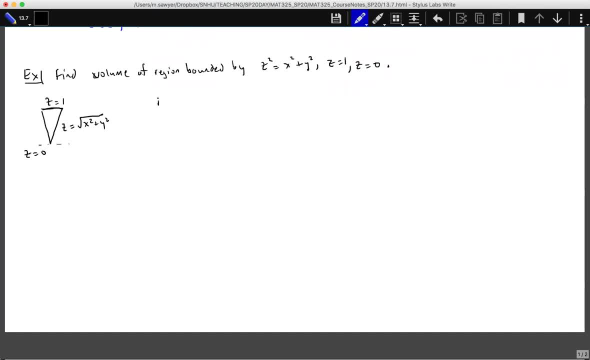 looking at this particular function, we know that R squared in cylindrical coordinates equals x squared plus y squared, so we can bound z. we think about our rectangles going from the line z equals square root of x squared plus y squared. think about our rectangles looking this way. we can say that z actually goes from R R squared. 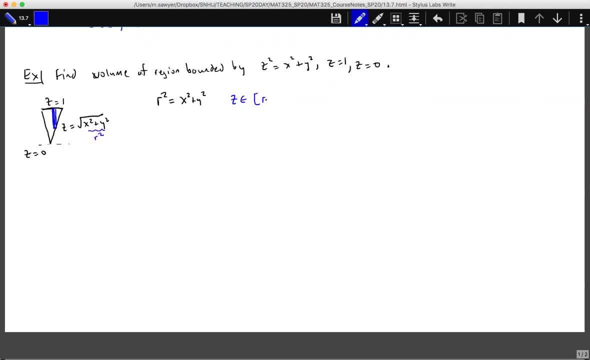 this piece here becomes R squared. z is equal to R, goes from R to 1, and since he starts at 0, that means that R goes from 0 to 1, and since we're looking all the way around, we have that theta has to go from. 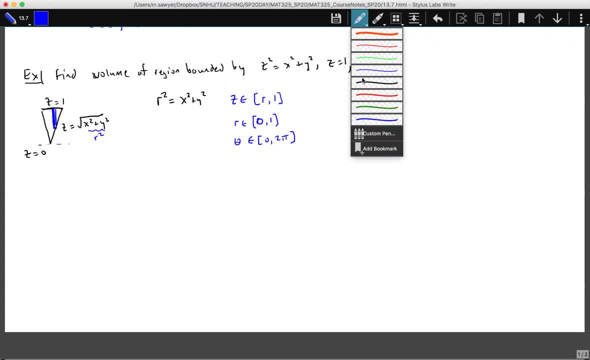 0 to 2 pi. so, setting up this integral, we have 0 to 2 pi, 0 to 1, R to 1 of R, dz, dr, d theta. we have no density function, so we assume the density is 1, so 0 to 2 pi and 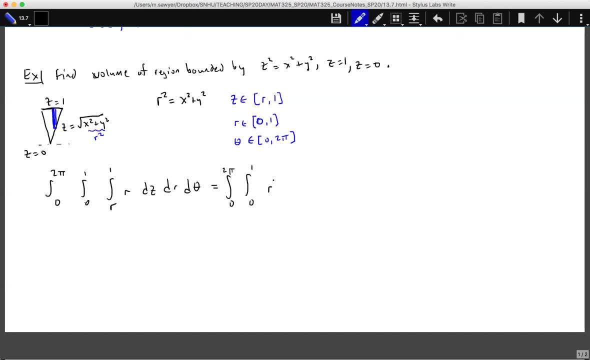 0 to 2 pi times R through z to equal 0 to 1. 0 to 1 of R minus R, R minus R- R squared dr theta. so this gives us 0 to 2 pi of 1 1⁄2 minus 1 th dt, which gives us 0 to 2 piifica1⁄3 dth. activity distance from 0.1 pi by 0.Ф T T. 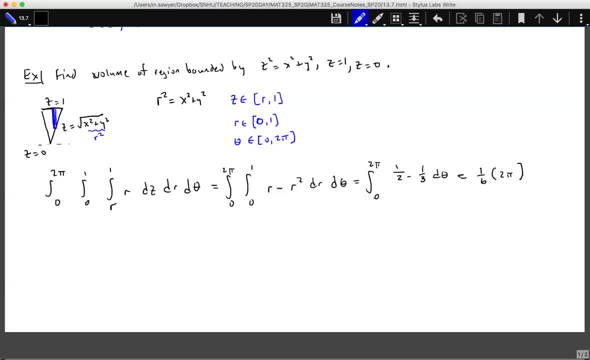 1, 6 times 2 pi, which gives us pi over 3 as the area of this chunk of the of the shape. and so it's important to note here that what we did is we turned our shape as to kind of this slice of a sphere, as a, into cylindrical coordinates and that 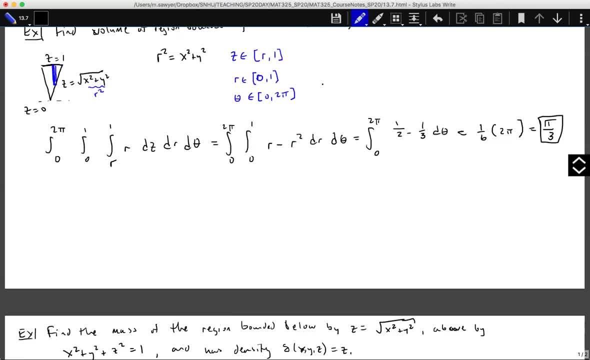 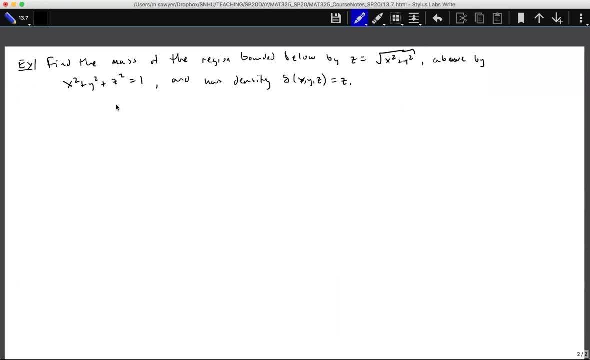 made our life a lot easier. so let's look at another example. let's find the mass of the region bounded below by this cone, the similar shape as we had before, and above by the top of the sphere. x squared plus y squared plus z squared equals 1. 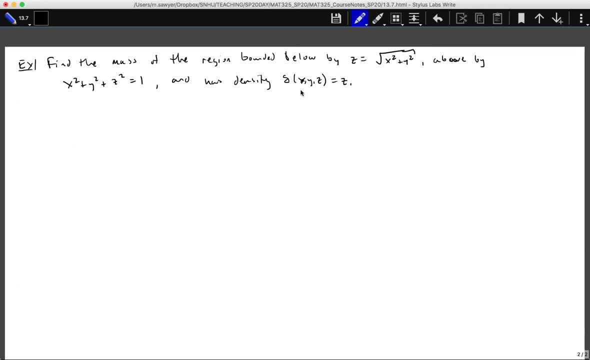 so this is a sphere with radius 1, with a density function. Delta of XYZ equals Z. so when we start dealing with spheres, this looks like perhaps an option to use spherical coordinates. so x squared plus y squared plus z squared is equal to Rho squared, so Rho equals 1. so we know that Rho is an upper bound here. so if we 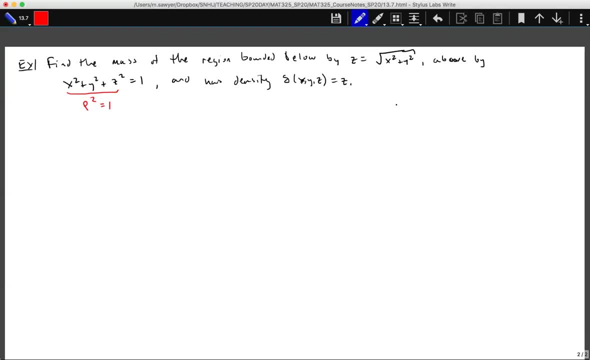 substitute in our- let's recall our- spherical coordinates. so X is equal to Rho sine of phi cosine of theta, Y is equal to Rho sine of phi, sine of theta, then Z is equal to Rho cosine of phi, and so when we're looking at this particular piece, we know that we 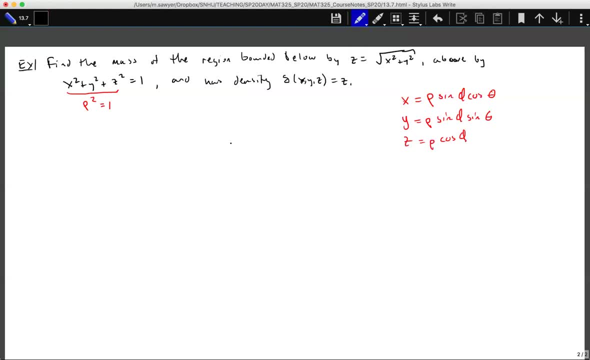 have x squared plus y squared equals plus z squared equals 1, is Rho squared equals 1 and then, if we take z squared is equal to x squared plus y squared, as our other bound from our other bound, so our, our lower bound, we can substitute in our definitions of our spherical coordinates. 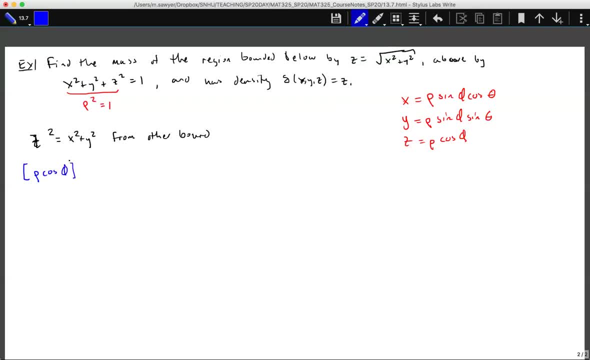 So z squared is equal to rho cosine of phi squared, and then x squared is rho sine of phi cosine theta squared, plus rho sine phi sine theta squared. So substituting in these pieces, so each piece will have a rho squared so we can divide through. 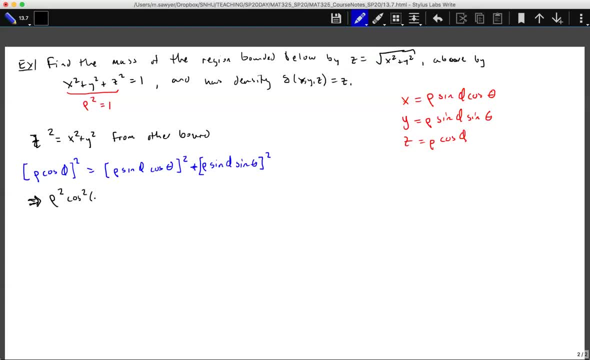 by the rho squared. but let's go ahead and see that precisely So: rho sine of phi. rho squared, cosine of squared of phi. rho squared sine squared of phi. So we can cancel out all the rho squareds and then we also see that cosine squared plus. 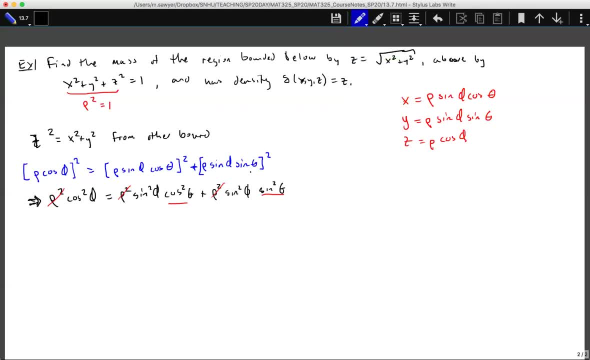 sine squared. we can factor out the sine squareds and we're left with: cosine squared of phi is equal to sine squared. So we could getaxisine squared of phi times cosine squared of theta plus sine squared of theta, but by our Pythagorean identity this piece is equal to one. 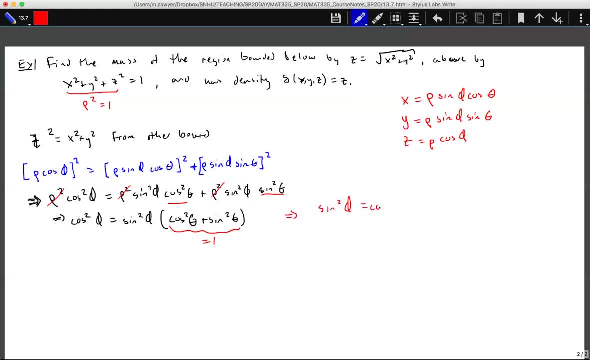 So this gives us that sine squared of phi equals cosine squared of phi, which means that tangent, if we divide both sines by cosine, tangent squared of phi equals one. 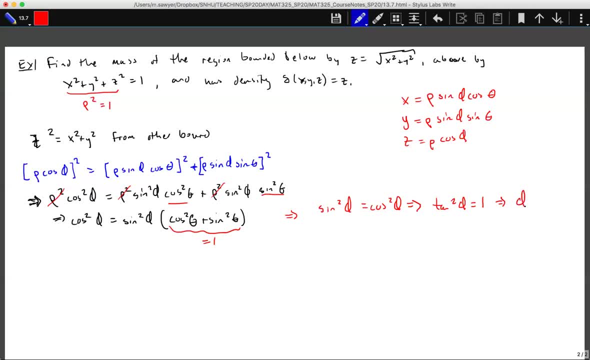 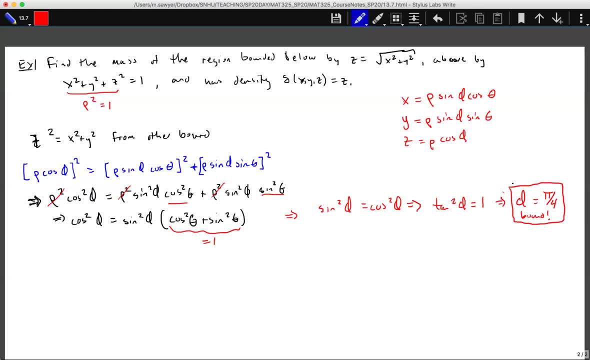 domain 0 to pi over 4, or 0 to pi for a domain, for phi means that pi over 4 is a bound, So this is helpful. So, since we're looking at the entire circle in the xy plane, we've got an idea of our 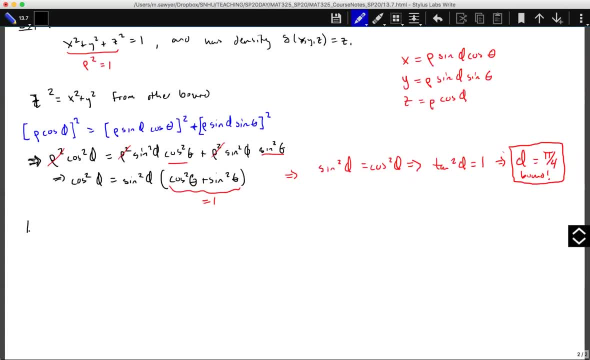 bounds here. So what we've done is we've used our bounds on the problem to develop our pounds on the interval. So we know our rho goes from 0 to 1.. We know our theta goes from 0 to 2 pi. since we're 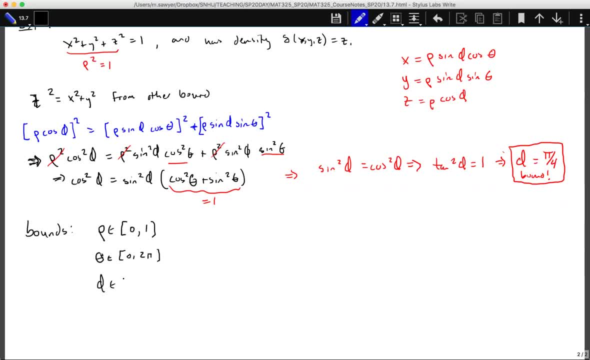 going around the entire sphere And our phi goes from 0, our lower bound. we're starting at the top of the sphere And we're angling down to pi over 4. And we can think of this. this actually looks like an ice. 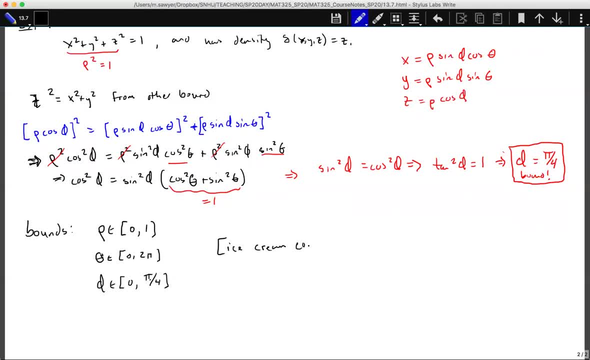 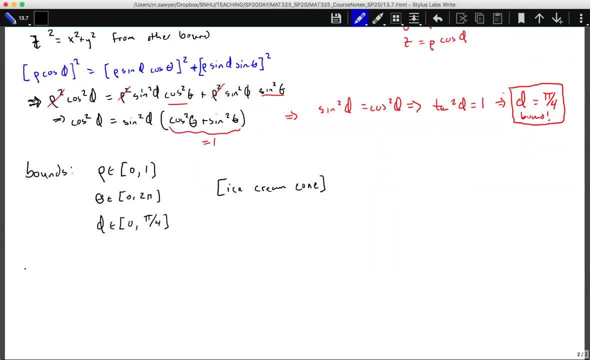 cream cone. So we have the cone on the bottom and the ball of ice cream on the top. So, as we're integrating this, we have 0 to 2 pi, 0 to pi over 4, 0 to 1.. 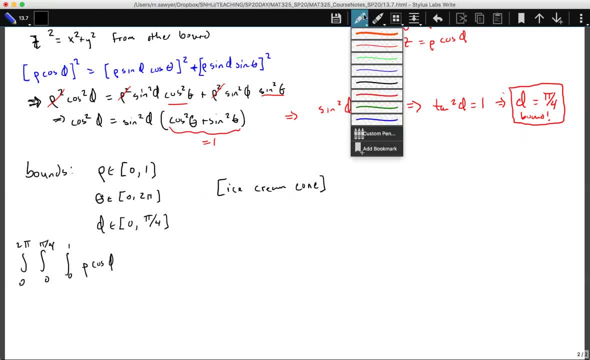 We're going around and we're going to multiply this by 2 and we're going to get the кв. So we want to make sure we keep it all in the correct coordinate system times, or Jacobian rho. squared sine of c. do you row the fee d theta so theta doesn't show up anywhere else in this problem, so we can pull out the two theta and theta. 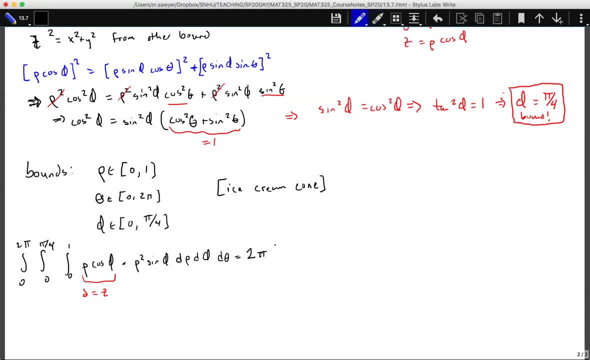 for the 2 pi. it's separable, so we can pull the theta all the way out front. this comes from our theta bounds, so this is as if we were to evaluate the outermost integral, because there's no thetas. this is all a constant in the 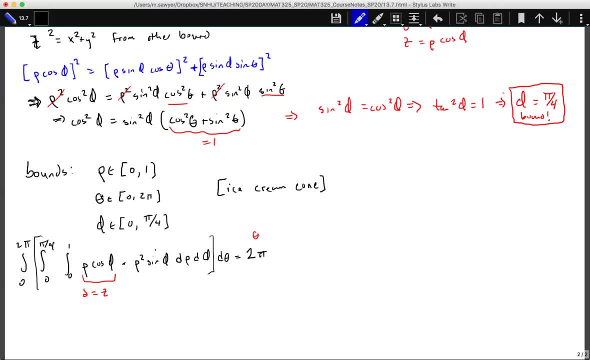 inside with respect to theta, so we can solve all this inside piece. and then we know the theta bounds is 2 pi. so versus we can't do it with Rho, because Rho shows up in the problem and Phi shows up in the problem, so those pieces may.